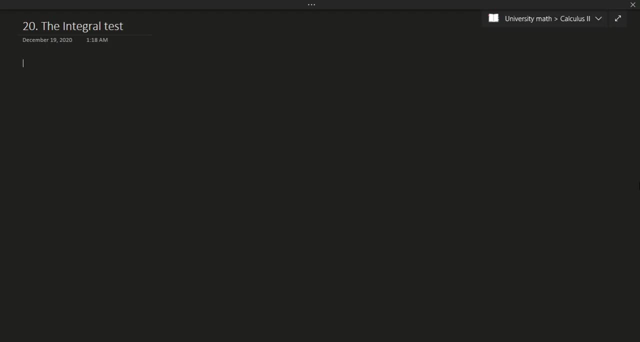 divergence of an infinite series. So let's talk about how this works. So here's the definition of the test in question. So suppose that f of x is a continuous positive. so these are important because they're actually kind of relevant to this test and a decreasing function. So decreasing. 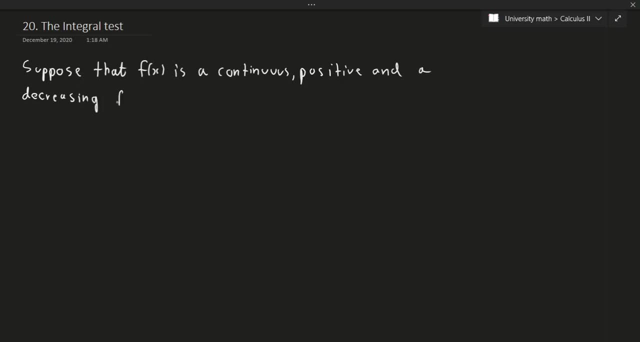 function. Notice I said function, not sequence, that's important On the interval k to infinity. and then, of course, notice that the key is in square brackets, so we include it, And f of x is a continuous positive. so these are important because they're actually kind of relevant. 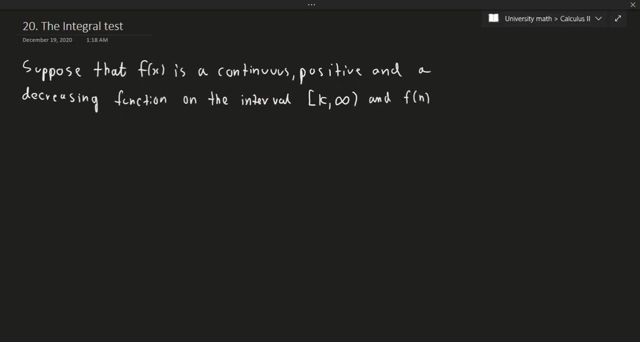 to this test. And then f of n is equal to a n. So basically I'm just saying that or not f of n, f of x is equal to a n. So basically I'm choosing the function so that it's equal to the series. it's equal to the series I'm evaluating, Okay. so here's the actual test. 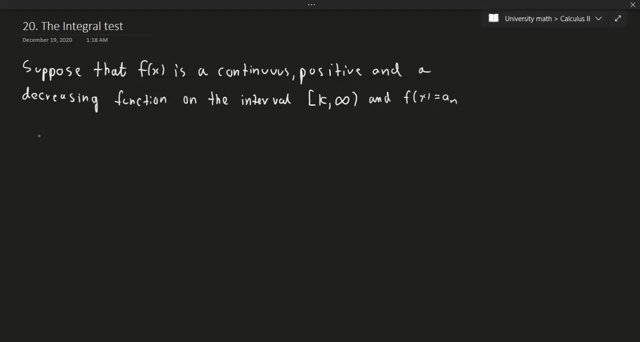 let me actually put this in green because it's kind of important. So if the integral from k to infinity, of f, of x times dx is convergent, then so is the following: So so is the summation from n equals k to infinity. 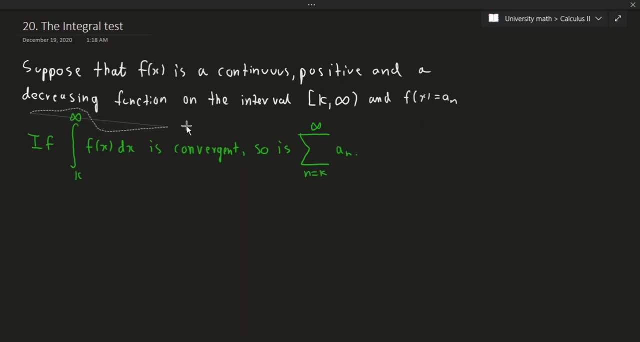 of a- n, we have a very similar kind of result for divergence. So I'm just going to copy paste that definition, because it's almost exactly the same thing. So here, if f of x is divergent, so in this case, if the integral of f of x- dx from k to infinity- is divergent, then so is 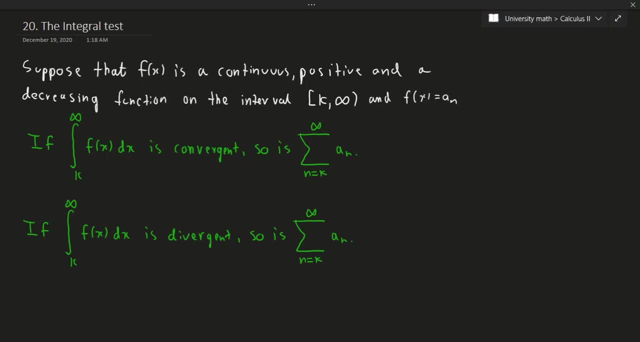 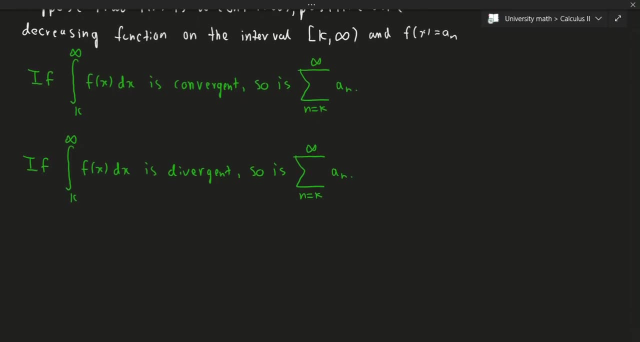 the sum in question. Okay, now here's a very important note I have to make, And I'm actually put this in red because it's actually very, very important. So let's just kind of write this down here: This sum- or let me correct that This doesn't need to be increasing or decreasing- 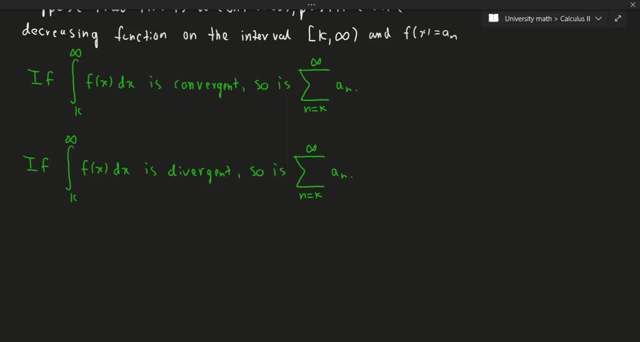 everywhere. It just has to be done in the long term. So what do I mean by that? I'm saying that initially it's possible that a sequence, or a series rather, can be increasing, But eventually, as long as it decreases in the long run. 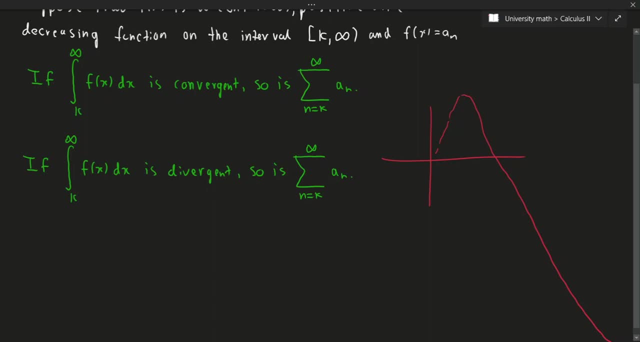 it will work out. So I don't really care what happens at the beginning, in the beginning of a series. it can oscillate back and forth however I want. It doesn't matter. What's more important is that eventually just kind of decreases at the end. So it's fine if it oscillates while back and forth. 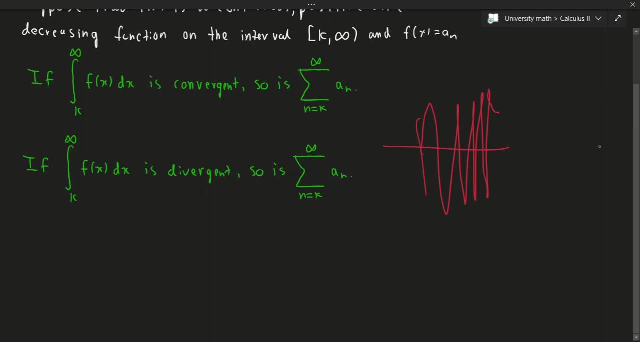 very widely, That's okay. What's important is that eventually it will sky down to zero, Unless you want to prove divergence in the case, and in that case it will just blow up like that: like sure, This part is fine. And if you want to prove divergence, as long as this happens in the 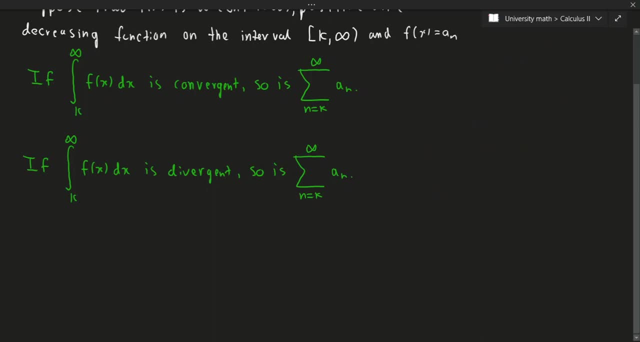 long term we're okay. But of course, generally you want to prove convergence. So the more important thing is that it's okay if it kind of blows up initially. As long as this eventually just kind of dies down to zero, we're okay. So you know, let's just go ahead and work with this. 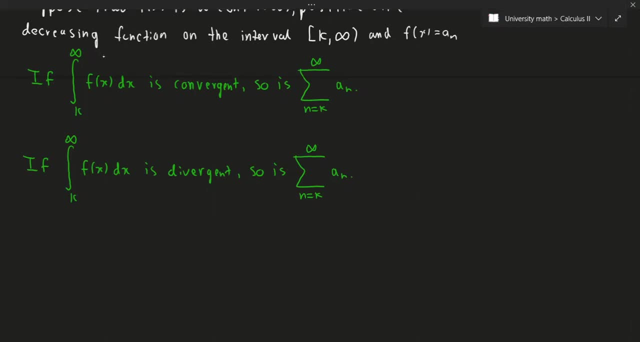 assumption and talk about how this works. I'm just gonna write this down first. So in this case, the sequence- or let me just not, let me not use sequence because that's wrong- The series does not need to increase or decrease everywhere. So I'm not saying, once again, it doesn't need to be increasing or decreasing. 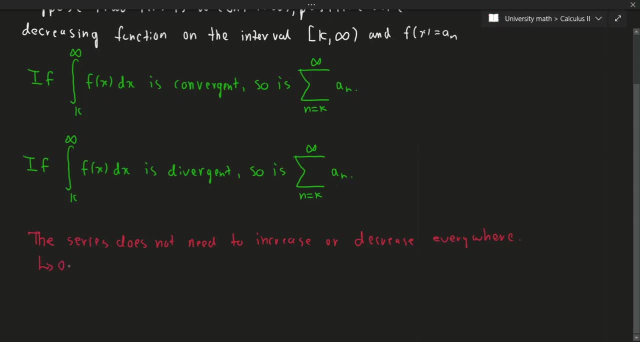 everywhere. It just has to do it in the long term, So only in the long term. We'll talk about what this means in a second. So let's kind of investigate for a second. Okay, so example: low zoom in. All right, here we go. 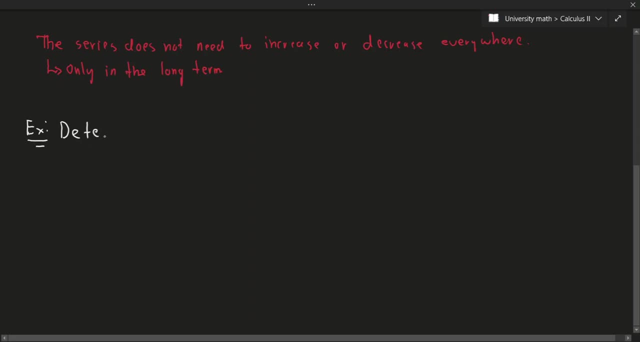 Okay, so determine if the summation from n equals two to infinity of one over n. natural log of n converges or diverges. Okay, here's the problem. We can use the geometric series or telescoping series on this, Because it's very hard to kind of recognize a pattern of sorts. 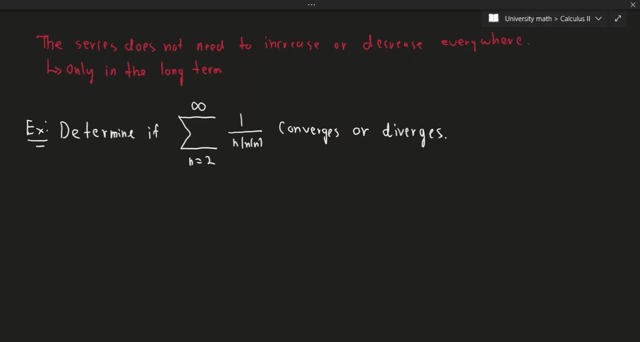 And there isn't any clever way we can use to manipulate the series to make it look like a telescoping series in any way. Nor is the geometric series- because it's not in the form ar- to the n minus one. So we can't really do anything about that And we can actually find a sum. But we can. 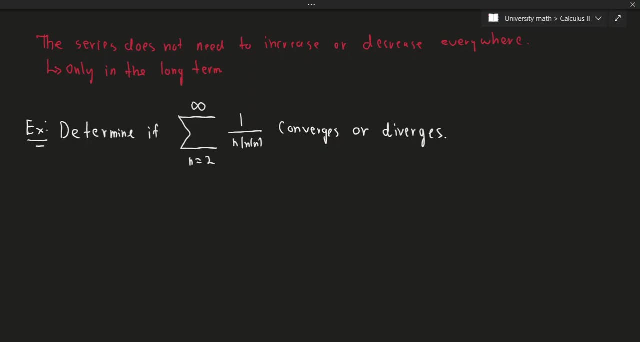 prove convergence or divergence using the integral test. So let's talk about how to actually do that. So let's take a look here. So suppose we have the summation from n equals 2 to infinity. So what we can do instead. 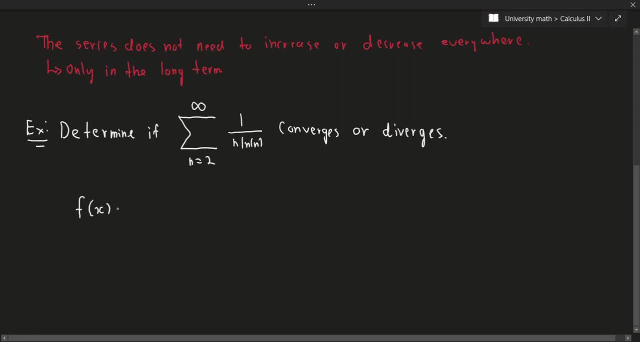 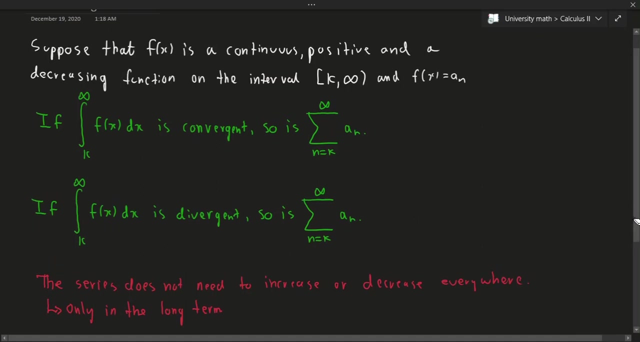 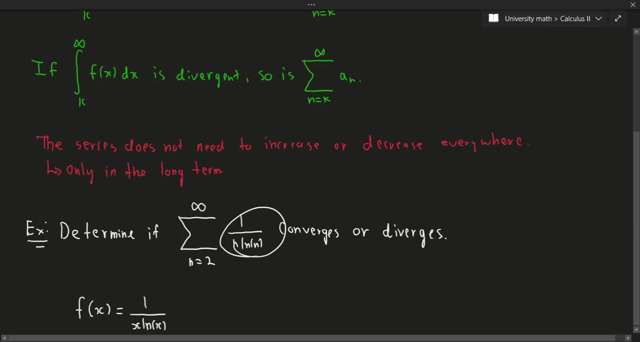 is, define a function f of x which is 1 over x times the natural log of x, And the reason I did that is because- let's take a look here- it needs to be a decreasing function In the summation. this was not a function, This is a sequence, So we can't quite use what we have in the series. 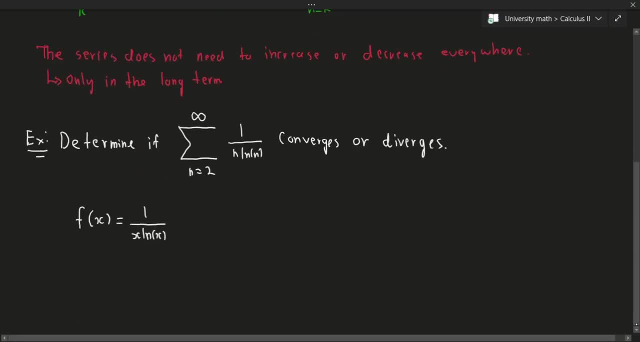 in order to use the integral test, And there's a very good reason for that. actually, The integral is a continuous set of values over an integral A series or, more appropriately, the sequence that I'm summing up is a set of discrete values, So you can't quite take the 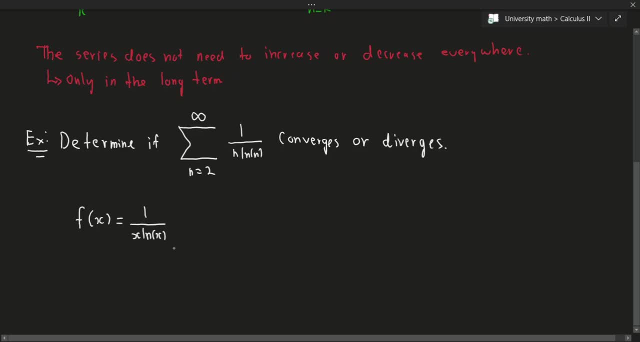 integral of a set of discrete values, So we have to use a function instead. Okay, now, that aside, we can now take the integral from 2 to infinity of 1 over x natural log of x times dx. Okay, this is just an improper integral, So we can now take the limit as t goes to infinity. 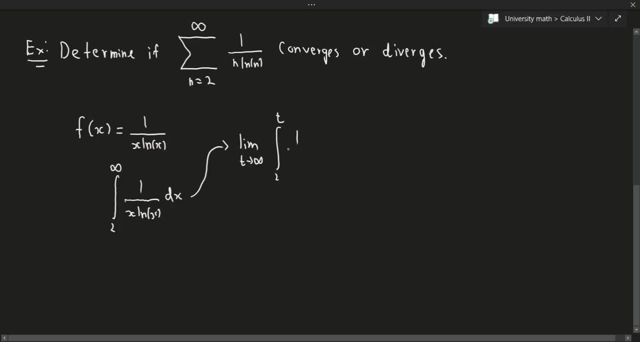 from 2 to t of 1 over x times the natural log of x. So we can now take the limit as t goes to infinity from 2 to infinity of 1 over x times dx. Okay, so what we can do is just kind of do this. 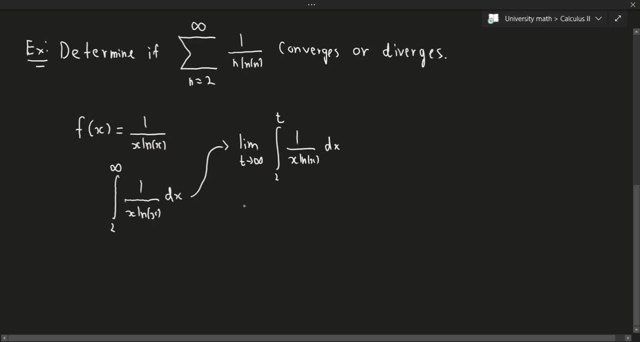 integral on the side. So I can just take the integral of this using a derivative. So u equals the natural log of x, du equals 1 over x times dx. So that means well, this is going to give us the integral of 1 over u times du, And that's going to give us the natural log of u plus a. 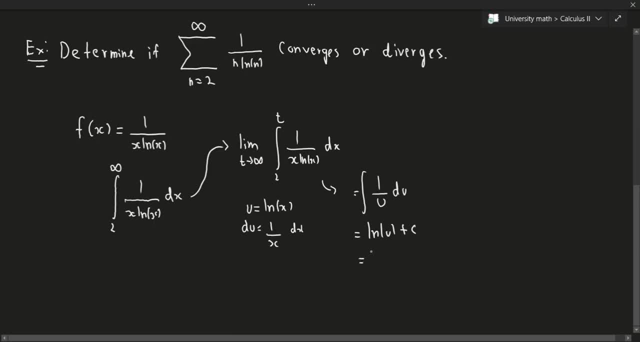 constant. But then of course u equals natural log of x. So we get the natural log of the natural log of x plus a constant. So that is the indefinite integral. So what we can do now is do the definite integral, So we get the limit, as t approaches infinity, of the natural log of x. 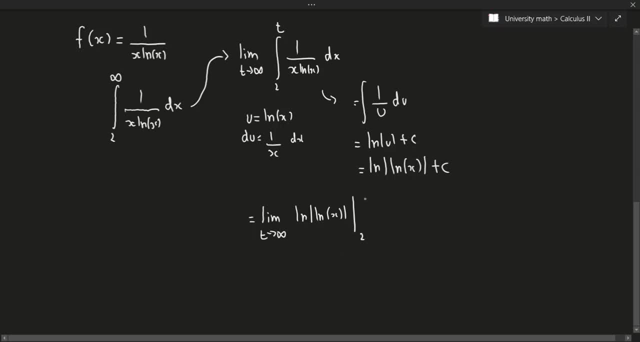 from, let's see, 2 to t, And then, if you go ahead and evaluate the integral, we'll get the limit, as t approaches infinity, of natural log, and we should probably keep the absolute value of the natural log of t, And we should probably keep the absolute value here as well. Actually, no, here we 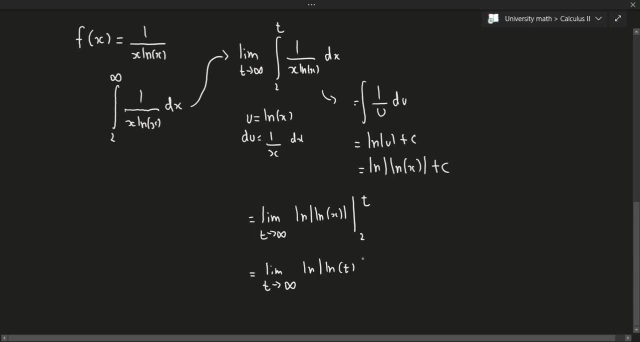 don't need to. Let's see, Minus the natural log of the natural log. Well, once we get the integral of 2. Like so Okay, well, if I take the limit to infinity, this thing is just going to blow. 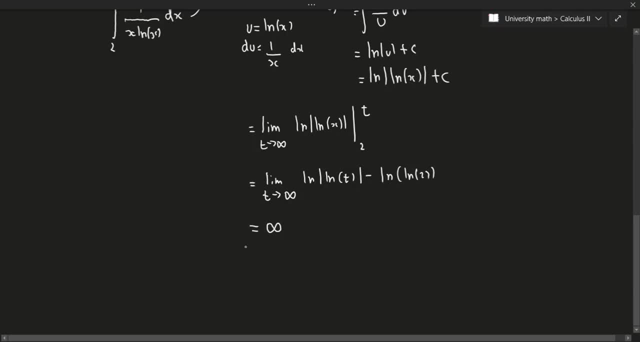 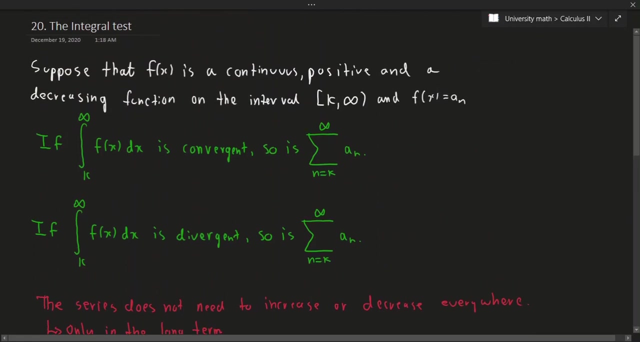 up. So this is going to go to infinity and therefore we can immediately conclude that this series diverges. So this is divergent, So nothing too crazy. So why could we use this test? Well, remember, this has to be a decreasing function and 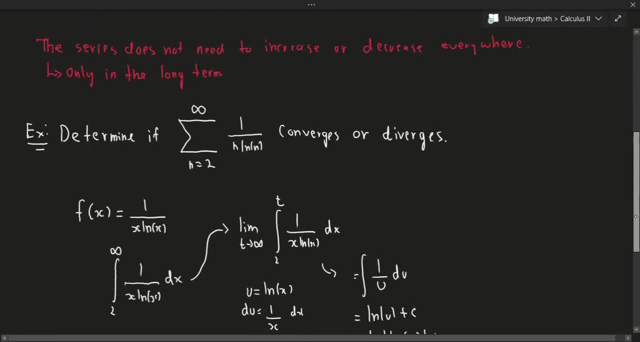 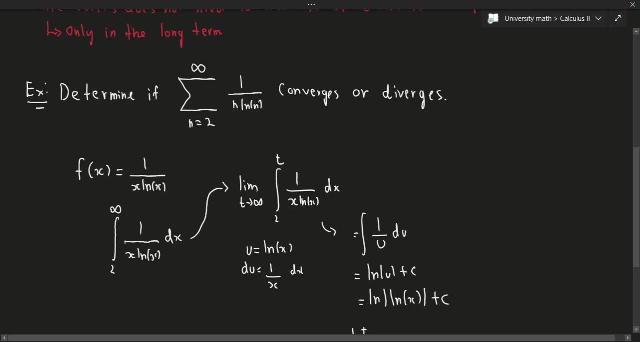 the integral has to exist for this to be convergent. Hopefully, you recognize that this was decreasing, because for larger and larger values, this is clearly a decreasing function. However, it won't always be that obvious all the time, So let's talk about example, where it's a little less obvious. You 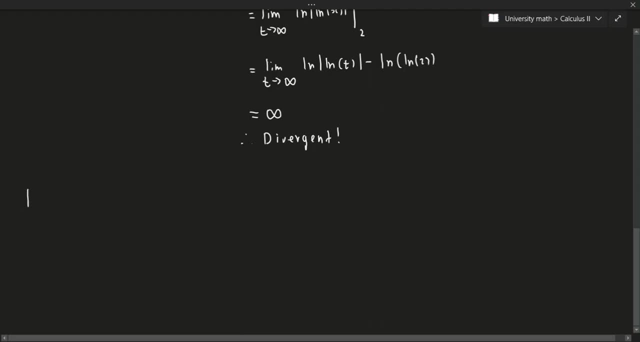 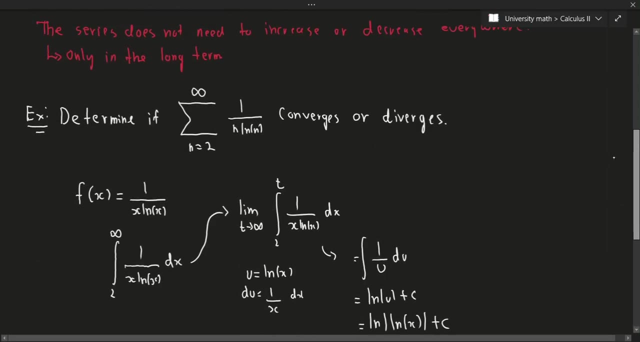 can still reason it out fairly easily. But I'm going to do an example of this. we have to vigorously prove this. So let's go ahead and do this out. So I'm going to copy paste the exact same question, but change the series. So let's go ahead and do that. 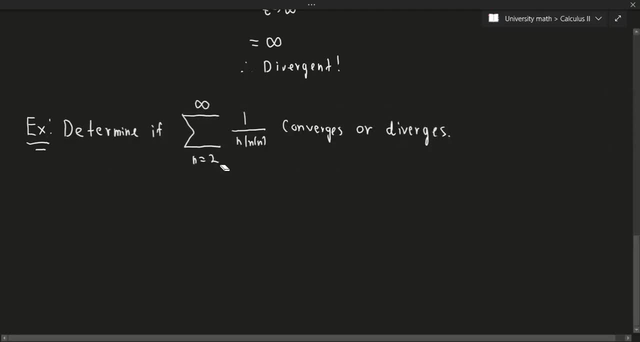 And here we go. So determine if the sum from n equals zero to infinity, of n, e to the minus n squared, converges or diverges. So once again, we can use the integral test on this. Well, that's the only test we've done so far, So we definitely know we have to use that one. 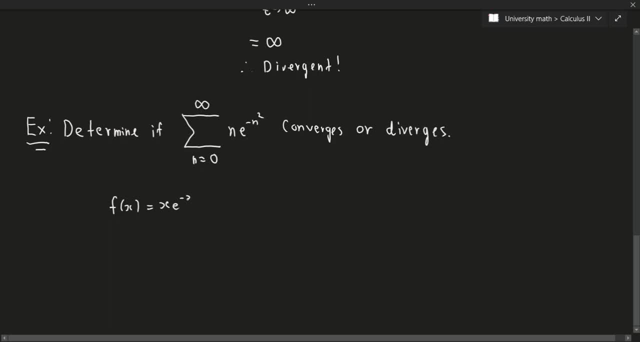 So, So, anyways. so in this case we'll get x. e to the minus x squared. We can rewrite this as x over e to the minus x squared, Okay, and then we can- oh, that should be e to the x squared. 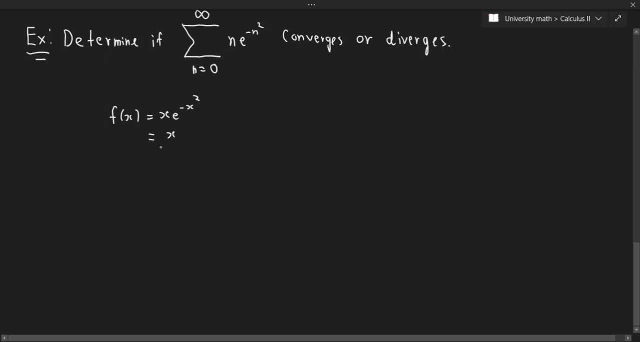 Now we could reason out that this is going to be decreasing because the exponential grows a lot quicker than a linear term. So yes, this is decreasing. But let's say we didn't know that. How would we prove that it's decreasing? 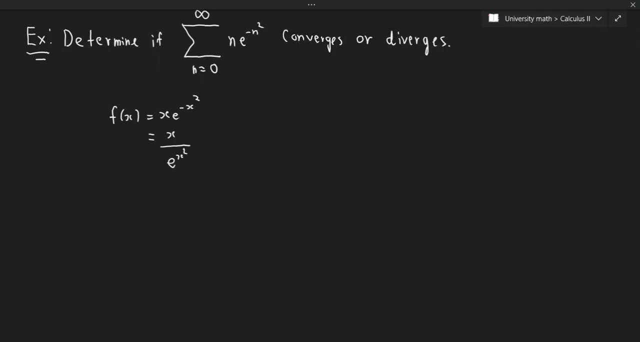 Well, one way we could do this is using calculus 1 knowledge. So we could take the derivative of this thing. So if we take the derivative, so f prime of x, I'm sure by now you know how to compute derivatives, So I will leave that step to you. 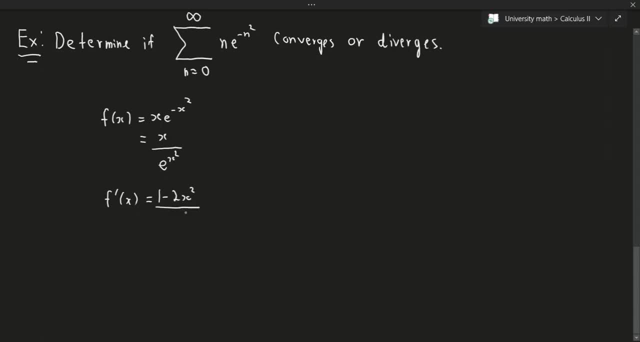 But if you go ahead and do this out, you'll get 1 minus 2x squared over e to the x squared, And that will be the result of the derivative. Okay, So now we need some critical points. So let's go ahead and find some critical points. 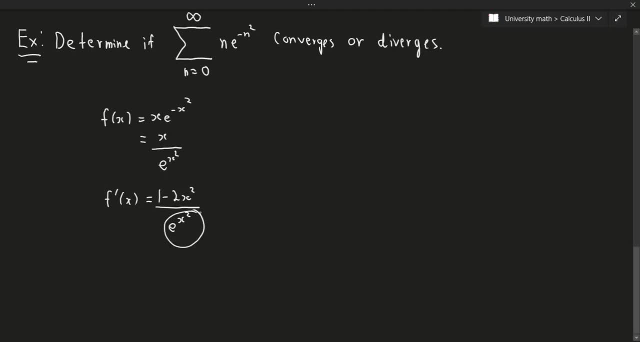 Technically we have to set this equal to 0.. But the exponential itself is never 0. So the denominator cannot be used to find critical points, But we can do it using a numerator. So 1 minus 2x squared is equal to 0.. 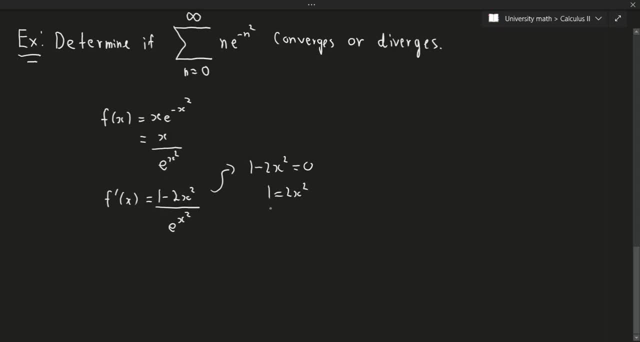 So 1 equals 2x squared, And then 1 over 2 equals x squared, Meaning that our critical points, our plus or minus 1 over the square root of 2 is equal to x. But here's the thing: This series goes from n equals 0 to infinity. 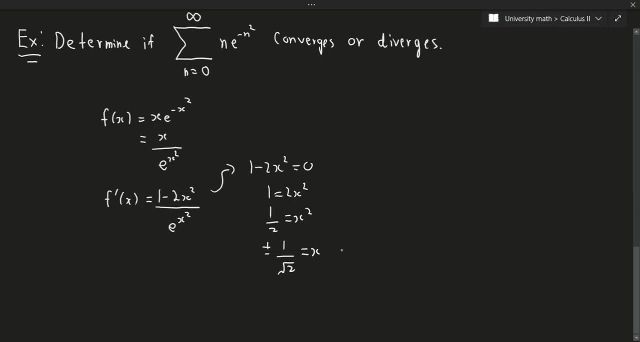 And then, because of that, we can kind of disregard the negative critical point. So our only useful critical point in this case is just 1 over 2.. Okay Now, with that being said, let's go ahead and plot in a number line to check what's going on. 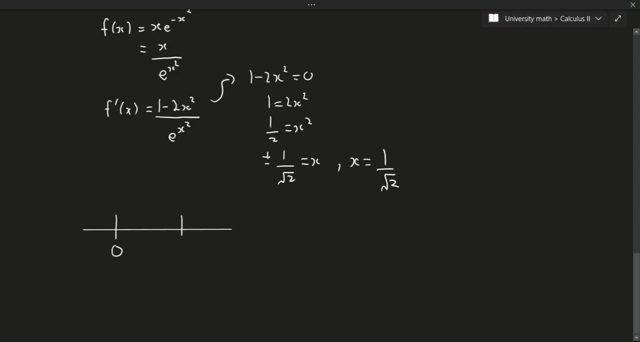 Because the series starts at 0, we have to use it. And then let's check what happens at 1 over root 2.. So we pick some test value, Like let's say so, a nice test value that we can use is the following: 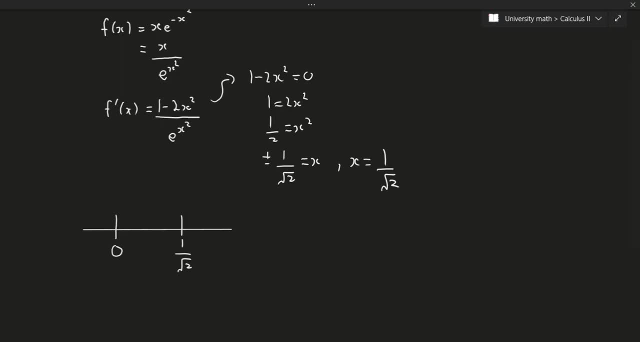 So 1 over root 2 is approximately 0.7.. So we could use, for example, 1 half as our test value And we could pick some like 5 for the higher value. But if you go ahead and test these values yourself, 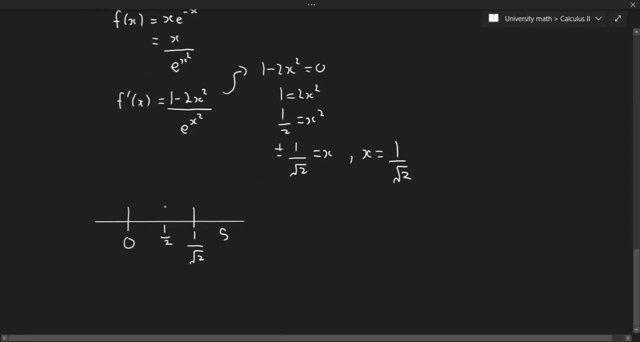 you'll see that this thing is increasing, So it's positive And this is decreasing, As I mentioned earlier, it's okay if this is initially increasing. What we care about is if it's decreasing in the long term, which it is. 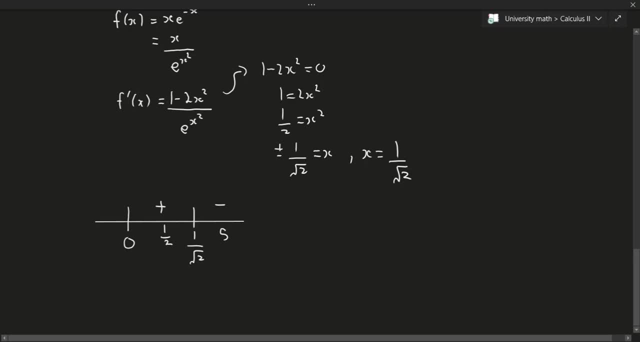 So from 1 half to infinity it's decreasing. So we don't really care about the fact that this is increasing in the first little bit. In the long term this barely matters, Kind of like the span of the human life and the age of the universe. 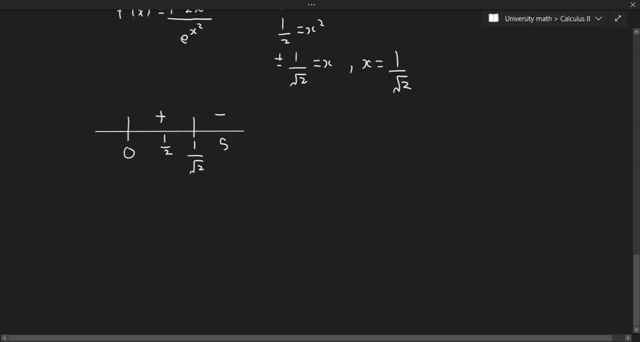 The age of the universe is like several billion years old, but humanity has been only around for like a few years. So to the universe we're like a speck of dust. This is how it feels to be working with series. Anyways, that was a bit on the side. 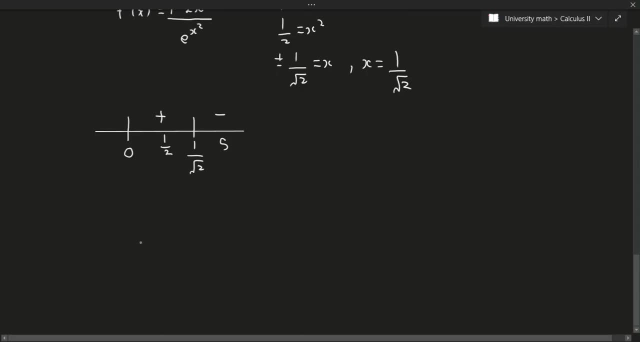 So let's keep going with this. So now let's go ahead and take the integral of this, So we get the integral from 0 to infinity, of x, e to the minus x squared times dx. Once again, this is an improper integral. 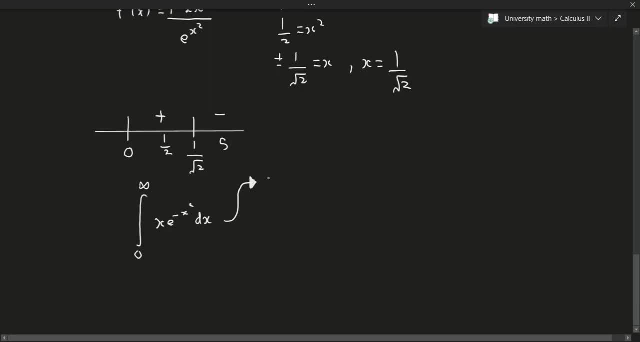 So we can go ahead and do a limit for this thing. So we're going to get the limit, As t approaches infinity, of the integral, from 0 to t, of x, e to the minus x squared times dx. To do this limit we can do a u, not the limit, the integral. 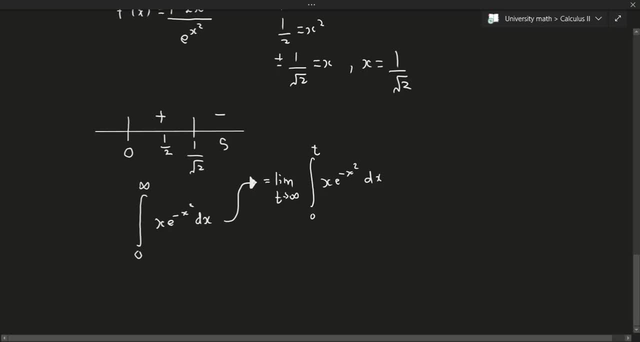 We can do a? u substitution, So we're just going to disregard the bounds for a bit. So I could let u equal to minus x squared. So du is equal to minus 2x times dx, Or minus 1 half times du equals x times dx. 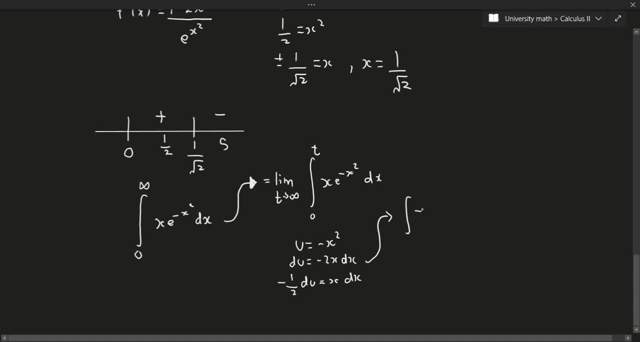 Meaning that our integral is going to become minus 1 over 2 e to the? u times du, Which is equal to minus 1 over 2 integral of e to the? u times du. Okay, well, if you take the integral of this thing, we get minus 1 over 2 e to the? u plus a constant. 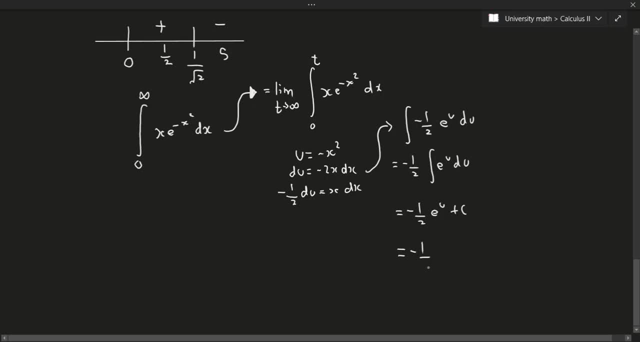 And then u is equal to minus x squared, So we get minus 1 over 2 e to the u times du, So we get minus 1 over 2 e to the minus x squared plus a constant. And then we can go back and do the limits. 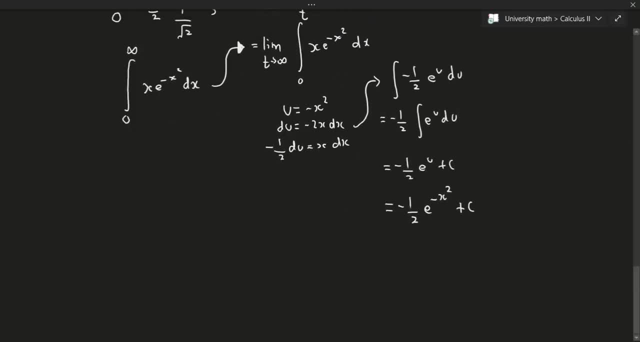 So when I say limits, I mean the bounds, And then we can take the limit as t goes to infinity. So if you go ahead and do this, we'll get the limit as t approaches infinity of minus 1 over 2 e to the minus x squared. 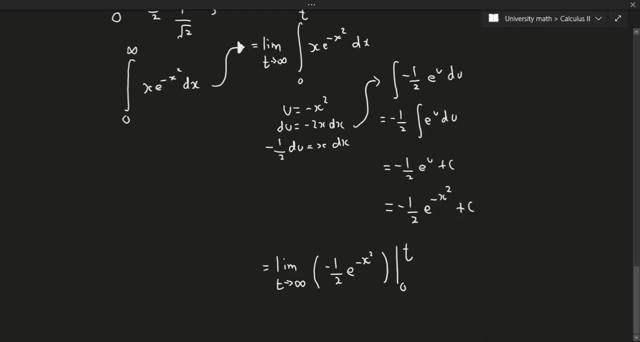 From 0 to t And then, if you go ahead and plug in the limit boundaries, we'll get the limit as t approaches infinity. And when I say the limit boundaries I mean these points, not this limit. I should probably say the integral bounds to make it more clear. 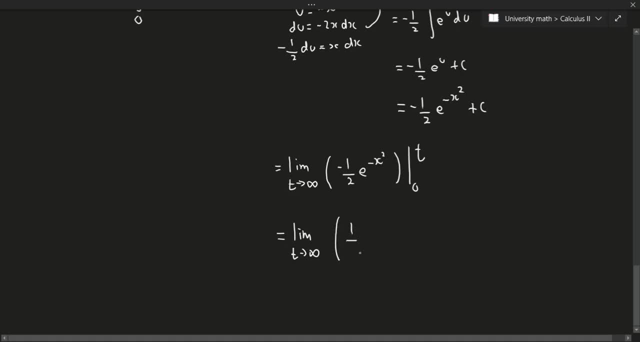 But nevertheless we're going to get 1 over 2, minus 1 over 2, e to the minus t squared, This thing is going to go to 0. Because it's a negative exponent. So finally, we'll just leave it 1 half. 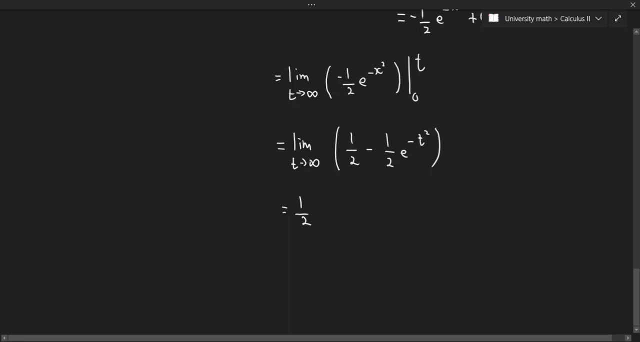 And because we get 1, half this thing is going to converge. So therefore, the series converges. So, once again, nothing very special going on here. Okay, Now here's a very interesting one, Because this, This one talks about a series we mentioned previously, in just a moment. 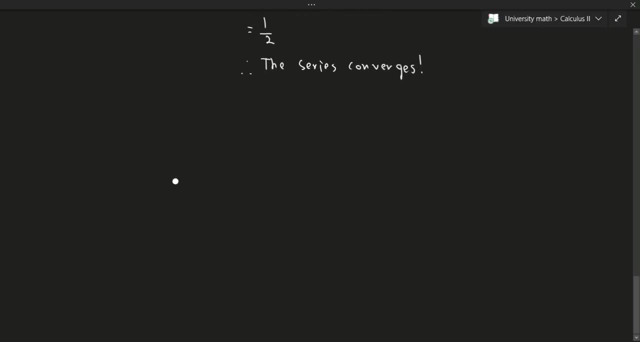 But we never really talked about why it worked the way it did. So let's go ahead and talk about this particular series. And what am I talking about? I'm talking about the harmonic series. So prove that, the harmonic series. So when I say the harmonic series, recall the harmonic series was the summation, from 1 to infinity, of 1 over n. 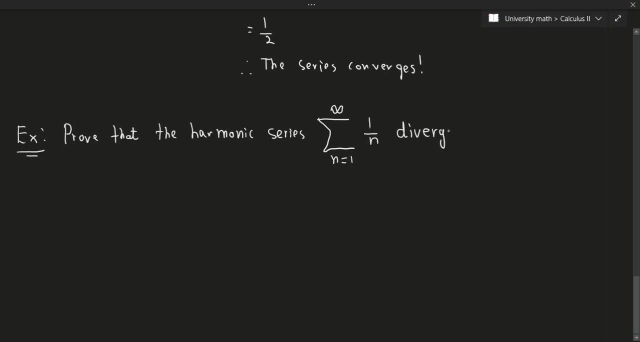 Prove that this series diverges. Okay Well, how does this work? Well, let's you know. take a look at this. Okay Well, first of all, we should probably check that. you know, We should probably rewrite this. 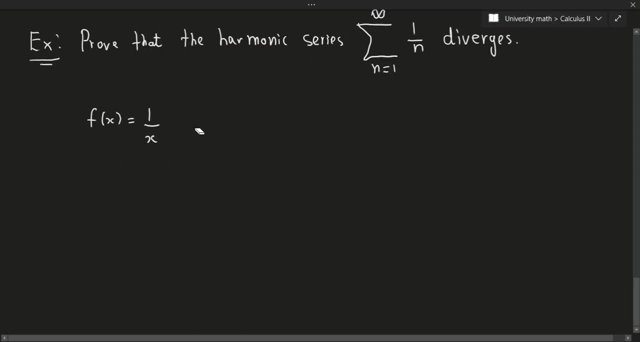 This is a function. I'm sure you don't need a PhD in math or anything to tell you that this is clearly a decreasing function. I mean, come on, This is clearly decreasing. So I mean, if you want, you can take the derivative and check the critical points. 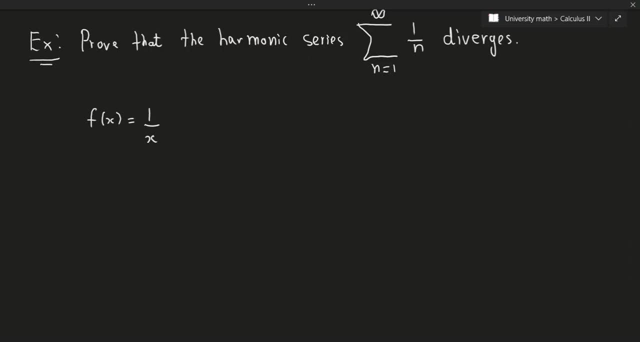 But there is literally no reason to do so. This is clearly a decreasing function. It's painfully obvious. So you know, let's go ahead and do the sum out now. So now we can go ahead and do the integral of this thing. 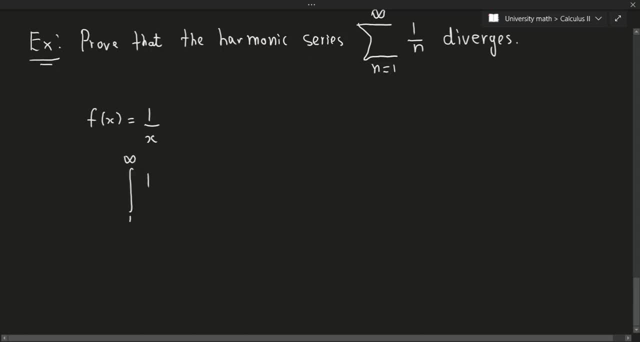 So we get the integral from 1 to infinity Of 1 over x times dx And then once again, just like the other kind of examples- and this will be the case pretty much all the time- we need to do a limit, because this is an improper integral. 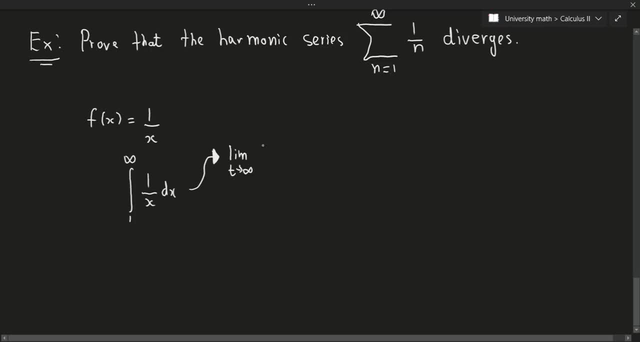 So we get the limit, as t approaches infinity, of 1 to t, of 1 over x times dx. We don't need to do any kind of fancy substitution for this. The integral of 1 over x is just the natural log of x and the absolute value of it, rather, 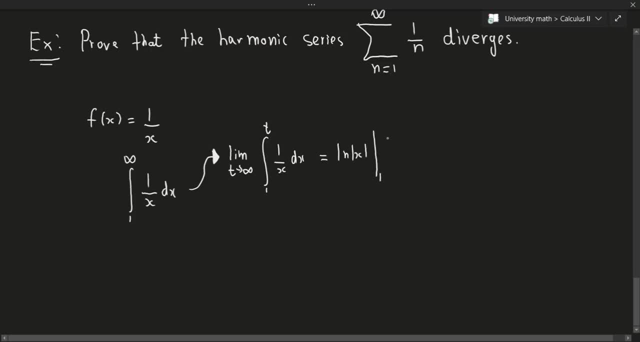 So we get the natural log of the absolute value of x from 1 to t, And we should probably do a limit of this thing, So let me just go ahead and put this on the side right here. So here we get the limit as t approaches infinity.